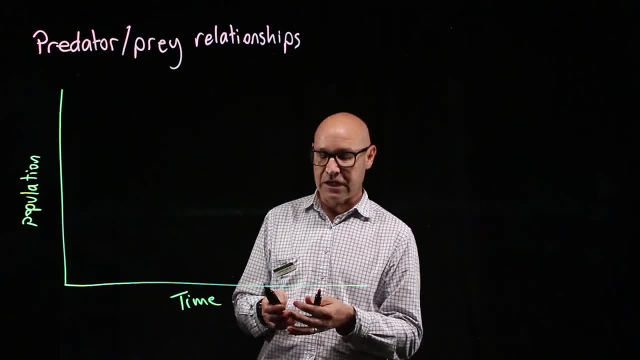 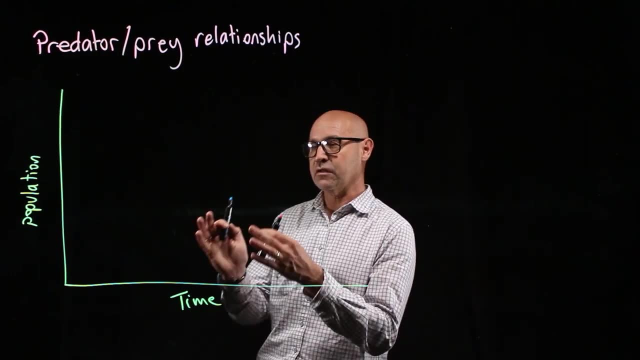 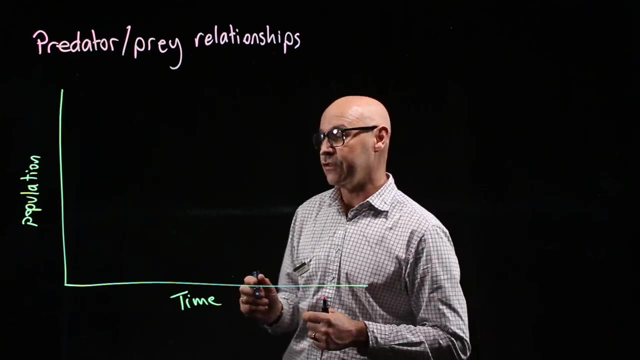 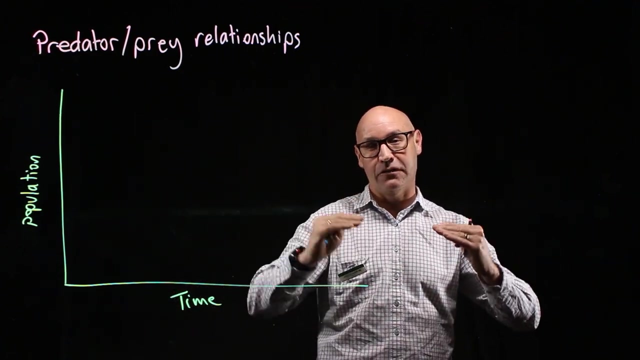 on the type of species. I want you to see that there's a relationship between the predator population and the prey population. So firstly, I'm going to start by drawing the start of the prey graph. So what we see with both species is the population cycles. They have booms and busts, The population. 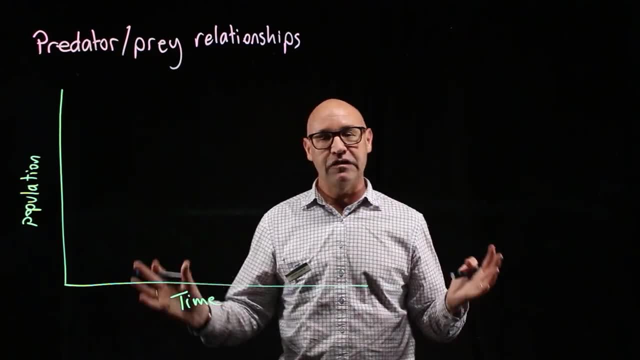 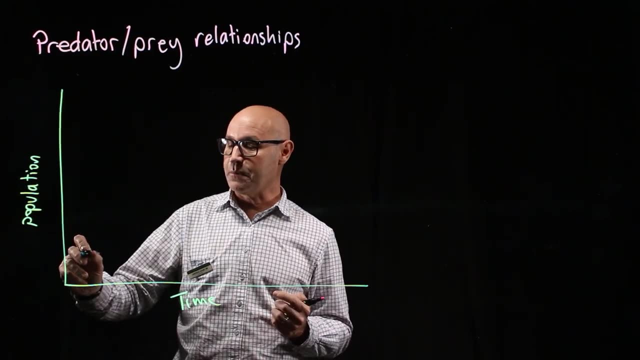 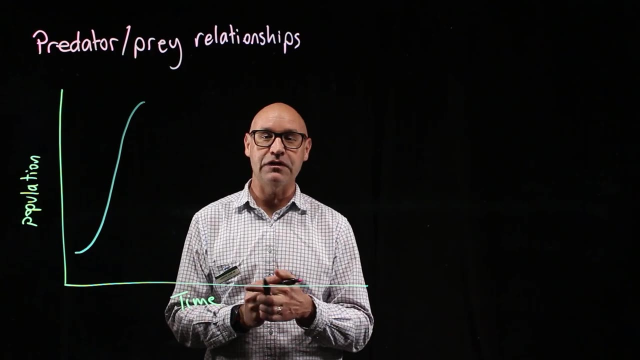 increases and then decreases. So when conditions are ideal for the prey- there's plenty of food, there's good environmental conditions for them to be able to reproduce- their population increases. But then it gets to a point where it can't increase anymore. It gets to what we call. 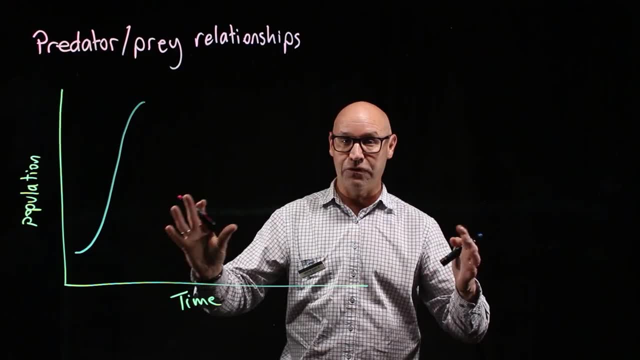 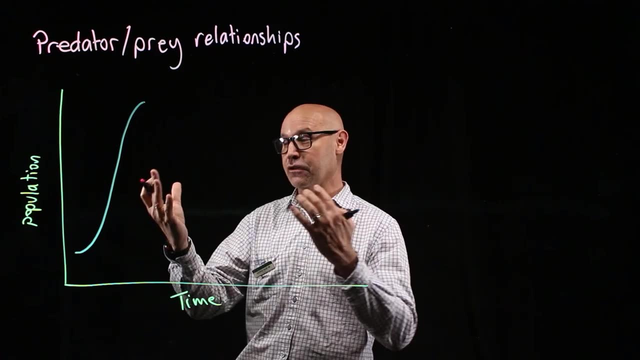 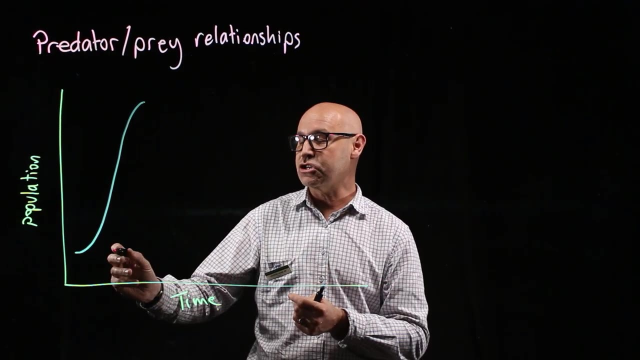 its carrying capacity because there's not enough food to sustain the population. Maybe there's the introduction of disease, or it's because there's so many prey organisms to eat. it attracts the predators. So the predator population then comes along and starts to increase to feed on those prey. 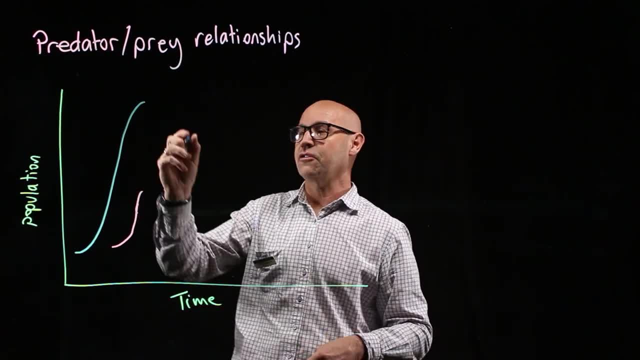 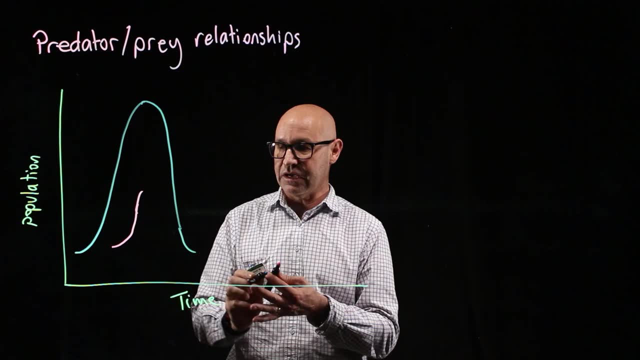 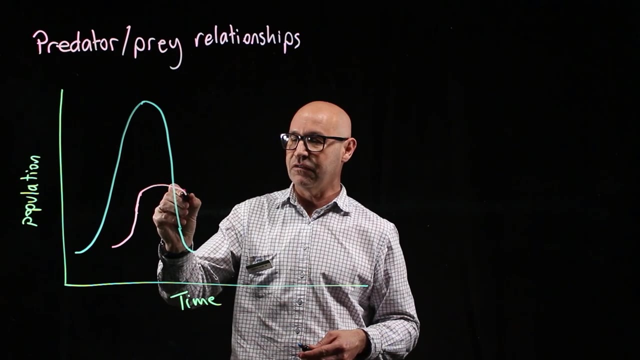 And, of course, if they're feeding on the prey, it's going to mean that the prey population is then going to decrease. So if the prey population decreases, that means that the same thing is going to happen with the predator population – it's also going to decrease. And if the predator population 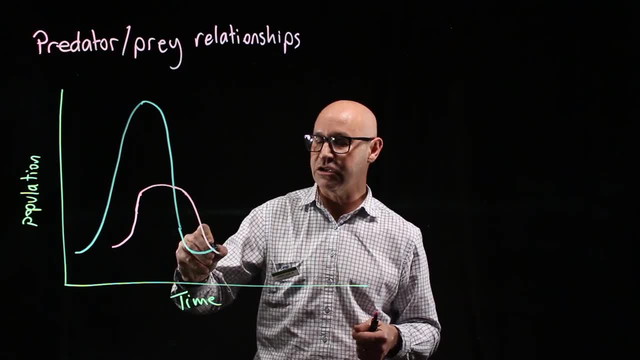 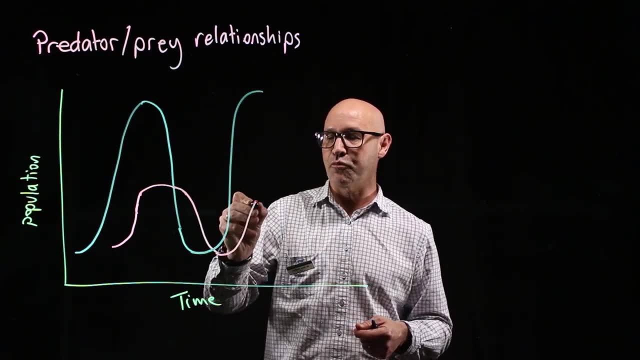 decreases, well then. well, that's the ideal time for the prey population to increase again. And if the prey population increases, well, that's going to be the ideal time for more predators to come along or reproduce and increase the predator population. 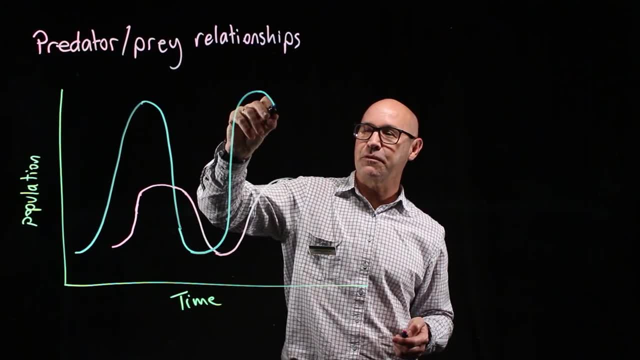 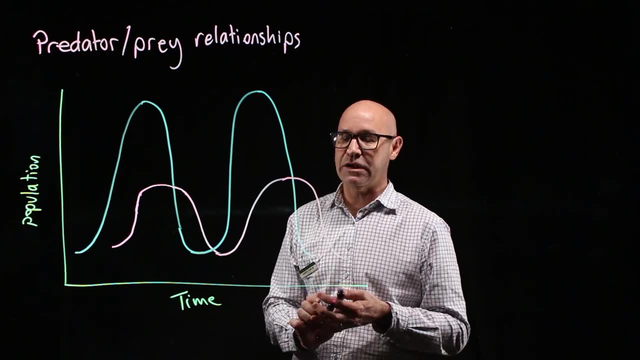 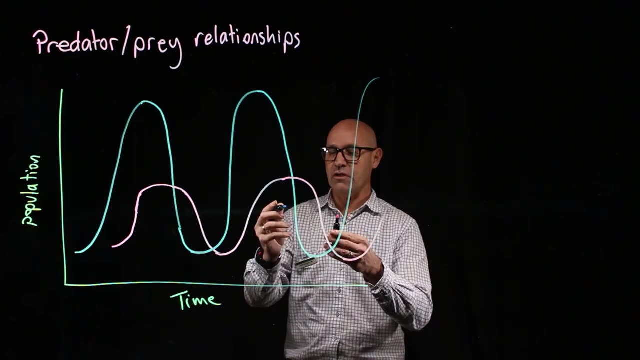 So then, if there's an increased predator population, then that means we're going to have a decrease in prey population, and then we're going to have the same pattern happen with the predators, and it's going to continue to cycle like that. Now I'm just going to go ahead and label this. 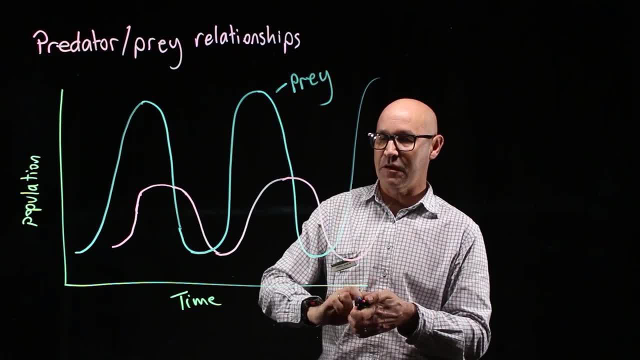 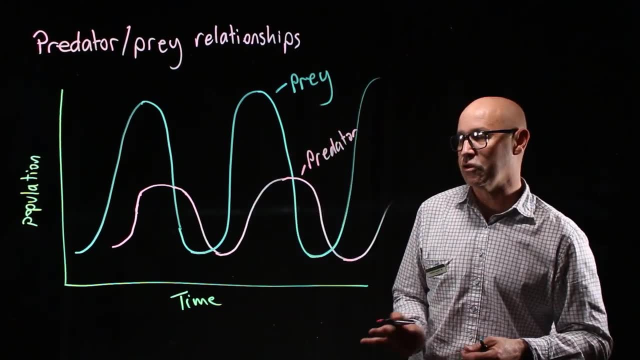 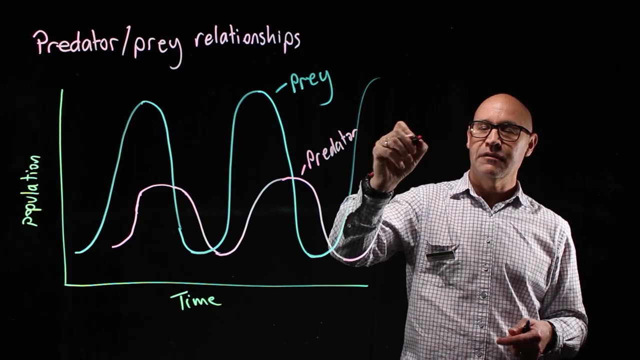 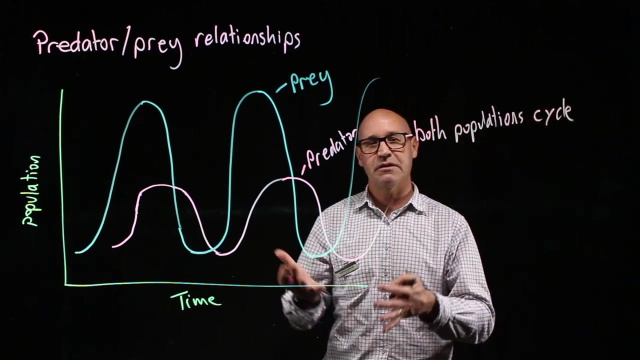 This is the prey and this is our predator population. Now there's a couple of observations I want you to make. Firstly, both populations cycle and they have the same pattern of boom and bust. So they both cycle up and down and boom and bust.